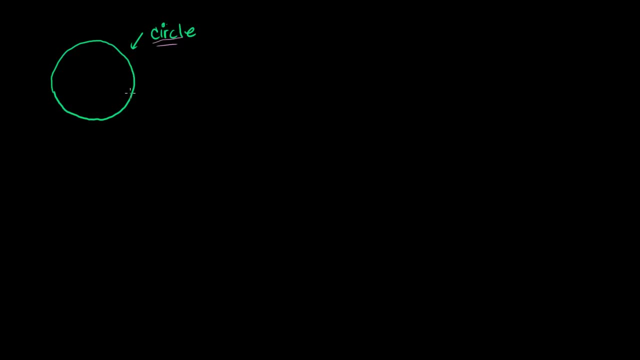 So it's probably worthwhile for us to understand some of the properties of the circle. So the first thing when people kind of discover the circle and you just have to look at the moon to see a circle- but the first time they say, well, what are the? 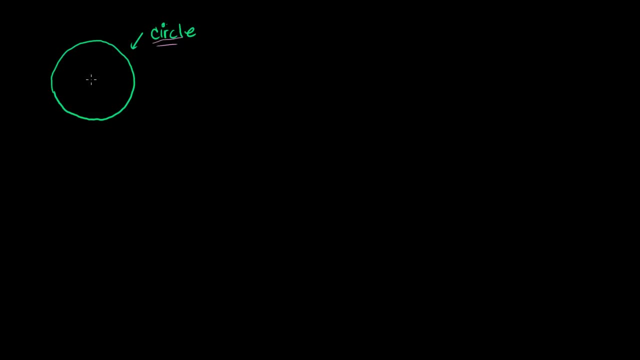 properties of any circle. So the first one they might want to say is: well, a circle is all of the points that are equal distance from the center of the circle, right. All of these points along the edge are equal distance from that center, right there. 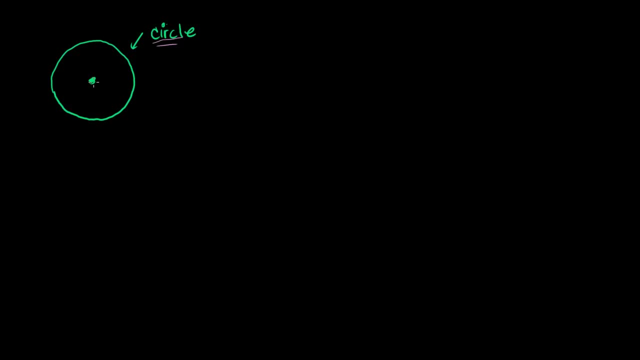 So one of the first things someone might want to ask is: what is that distance, that equal distance, that everything is from the center, right there? We call that the radius of the circle. It's just the distance from the center out to the edge. 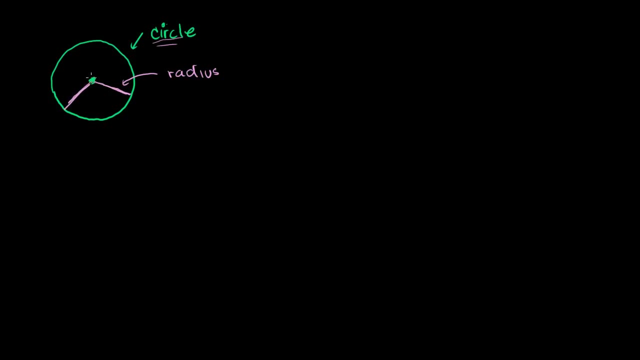 If that radius is 3 centimeters, then this radius is going to be 3 centimeters And this radius is going to be 3 centimeters. It's never going to change. By definition, a circle is all of the points that are. 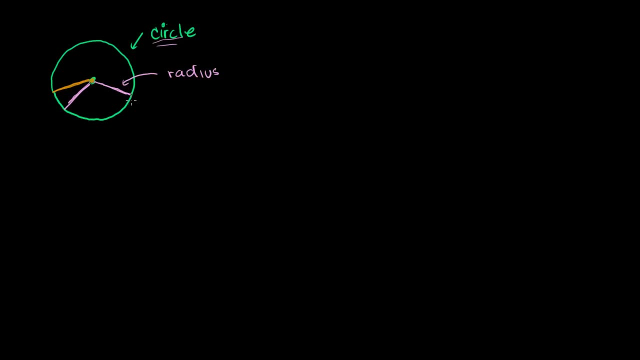 equidistant from the center point, And that distance is the radius. Now the next most interesting thing about that. people might say: well, how fat is the circle, How wide is it along its widest point? Or if you just want to cut it along its widest point, what? 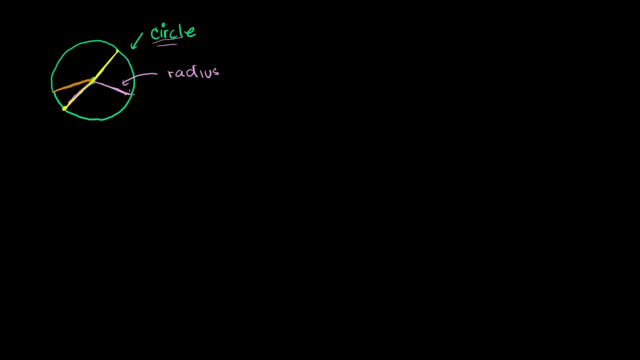 is that? What is that distance right there? And it doesn't have to be just right there. I could have just as easily cut it along its widest point right there. I just wouldn't be cutting it someplace like that, because that wouldn't be along its widest point. 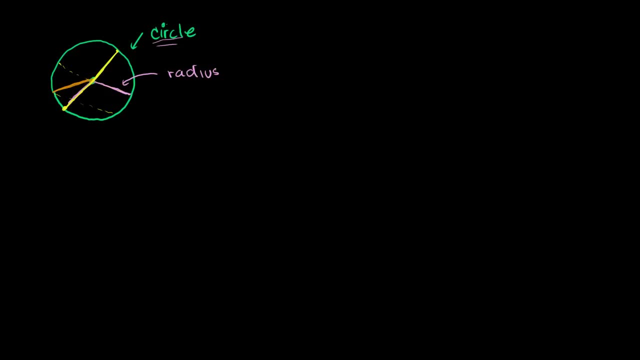 There's multiple places where I could cut it along its widest point. Well, we just saw the radius And we see that widest point goes through the center and just keeps going. So it's essentially two radii. You get one radius there and then you have another radius. 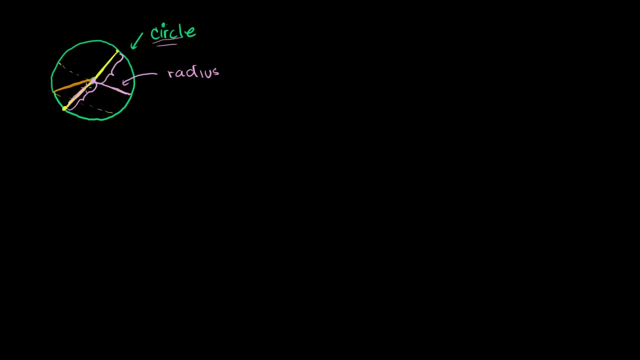 over there And we call this distance, Distance along the widest point of the circle, the diameter. So that is the diameter of the circle And it has a very easy relationship with the radius. The diameter is equal to 2 times the radius. 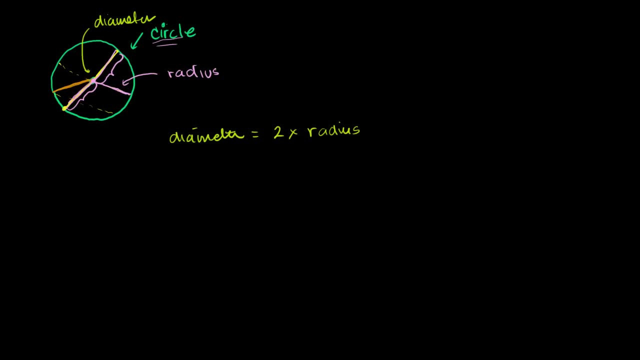 Now the next most interesting thing that you might be wondering about a circle is: how far is it around the circle? So if you were to get your tape measure out and you were to measure around, Around the circle like that, if you were to measure around, 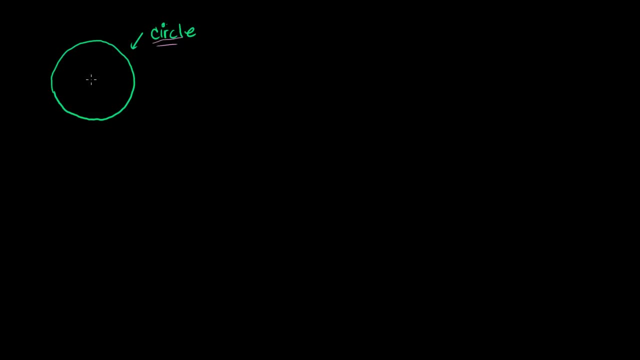 properties of any circle. So the first one they might want to say is: well, a circle is all of the points that are equal distance from the center of the circle, right. All of these points along the edge are equal distance from that center, right there. 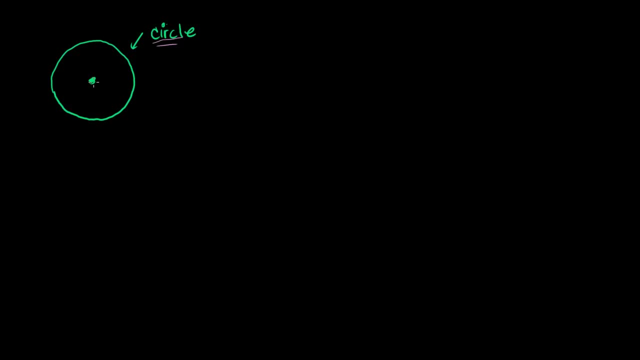 So one of the first things someone might want to ask is: what is that distance, that equal distance, that everything is from the center, right there? We call that the radius of the circle. It's just the distance from the center out to the edge. 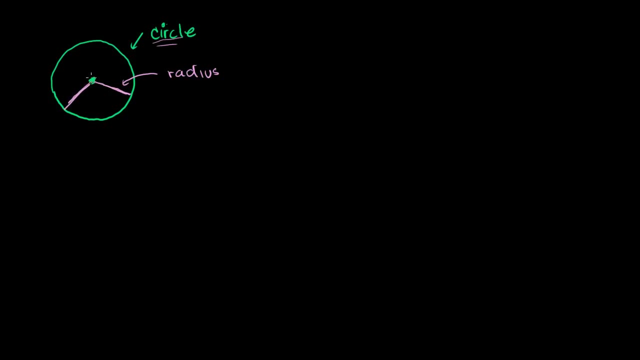 If that radius is 3 centimeters, then this radius is going to be 3 centimeters And this radius is going to be 3 centimeters. It's never going to change. By definition, a circle is all of the points that are. 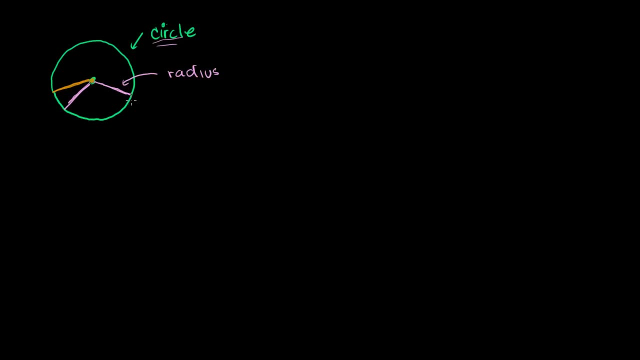 equidistant from the center point, And that distance is the radius. Now the next most interesting thing about that. people might say: well, how fat is the circle, How wide is it along its widest point? Or if you just want to cut it along its widest point, what? 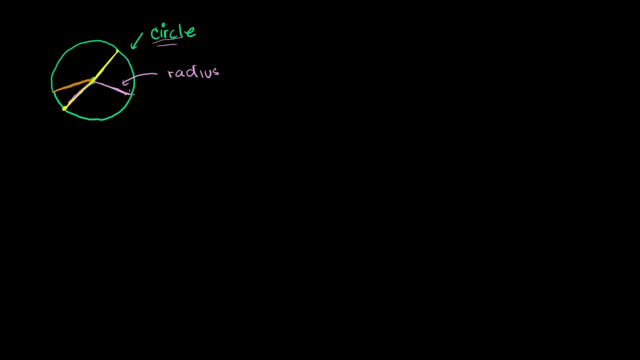 is that? What is that distance right there? And it doesn't have to be just right there. I could have just as easily cut it along its widest point right there. I just wouldn't be cutting it someplace like that, because that wouldn't be along its widest point. 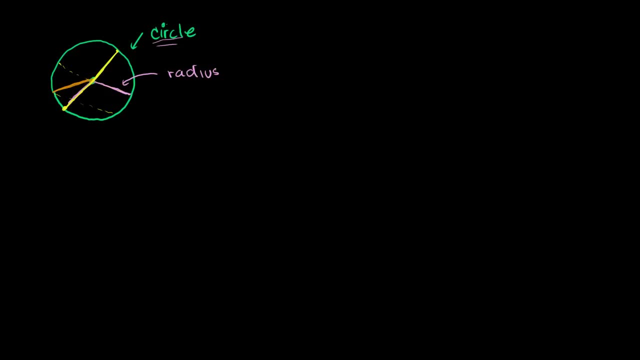 There's multiple places where I could cut it along its widest point. Well, we just saw the radius And we see that widest point goes through the center and just keeps going. So it's essentially two radii. You get one radius there and then you have another radius. 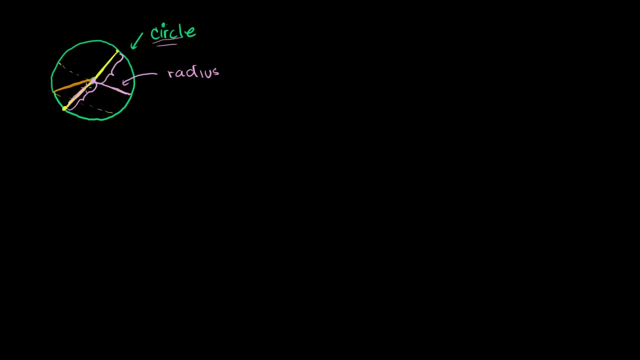 over there And we call this distance, Distance along the widest point of the circle, the diameter. So that is the diameter of the circle And it has a very easy relationship with the radius. The diameter is equal to 2 times the radius. 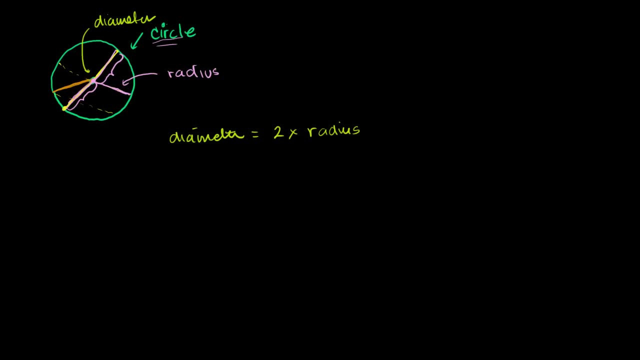 Now the next most interesting thing that you might be wondering about a circle is: how far is it around the circle? So if you were to get your tape measure out and you were to measure around, Around the circle like that, if you were to measure around, 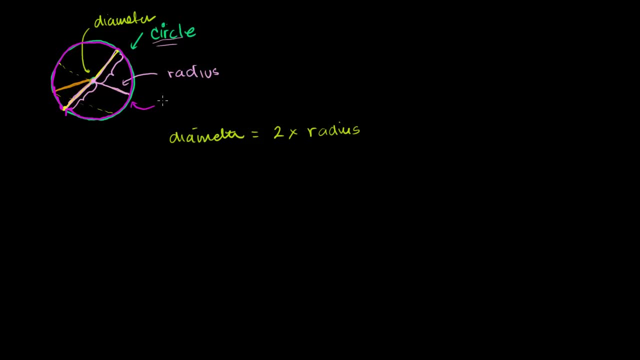 the circle like that. what's that distance? We call that word the circumference of the circle. Now we know how the diameter and the radius relates, But how does the circumference relate to, say, the diameter? If we know how it relates to the diameter, it's very easy. 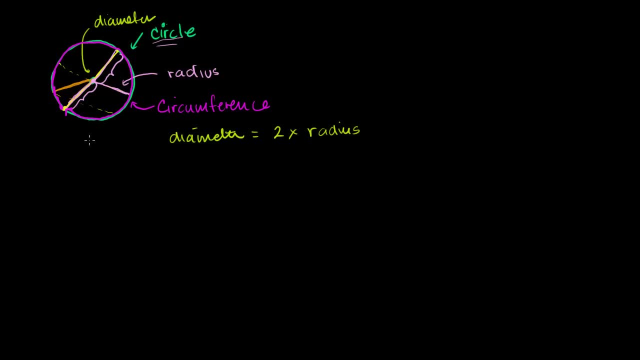 to figure out how it relates to the radius. Well, many thousands of years ago, people took their tape measures out And they keep measuring. They keep measuring circumferences and radiuses And, let's say, when their tape measures weren't so good. 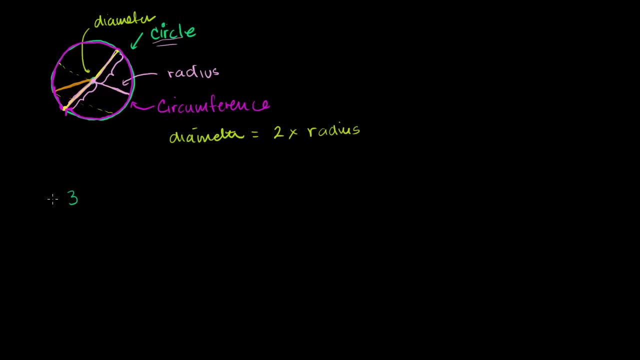 let's say they measured the circumference of the circle And they would get: well, it looks like it's about 3.. And then they measure the radius of this circle right here, or the diameter of that circle, And they'd say: well, that diameter looks. 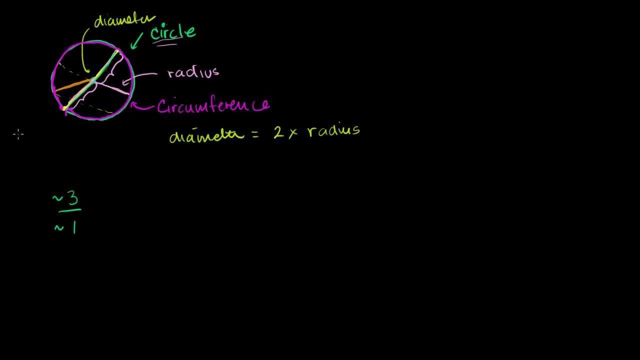 like it's about 1.. So they would say, let me write this down. So we're worried about the ratio of the circumference to the diameter. So let's say that somebody had some circle over here. Let's say they had this circle. 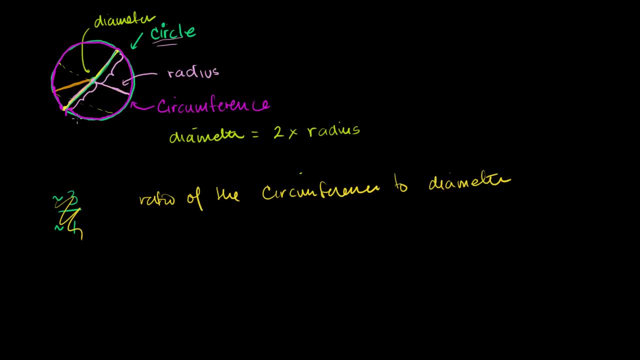 And the first time with not that good of a tape measure. they measured around the circle And they said: hey, it's roughly equal to 3 meters. when I go around it And when I measure the diameter of the circle, it's. 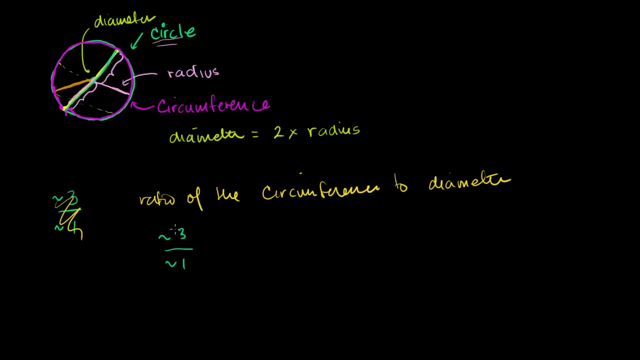 roughly equal to 1.. OK, that's interesting. It may be the ratio of the circle, The circumference of the diameter, is 3. So maybe the circumference is always 3 times the diameter. Well, that was just for this circle. 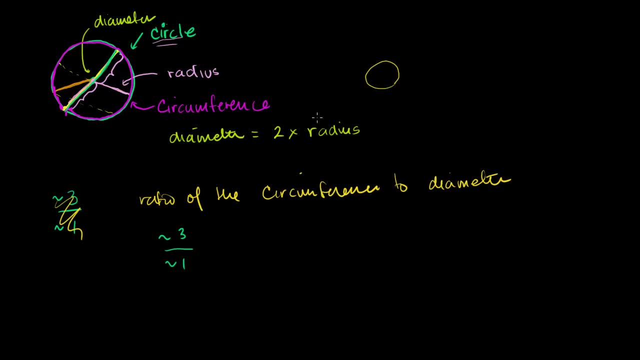 But then I'll say: they measured some other circle here. Let's say it's like this. I drew it smaller. But let's say that on this circle they measured around it and they found out that the circumference is 6 centimeters roughly. 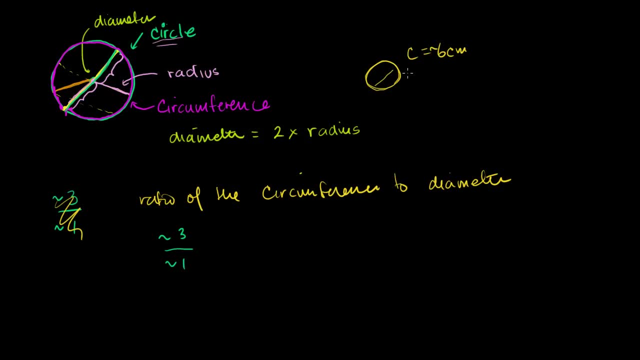 We have a bad tape measure right then. And then they find out that the diameter is roughly 2 centimeters And once again, the ratio of the circumference to the diameter, OK, The circumference to diameter was roughly 3.. So like, hey, this is a neat property of circles. 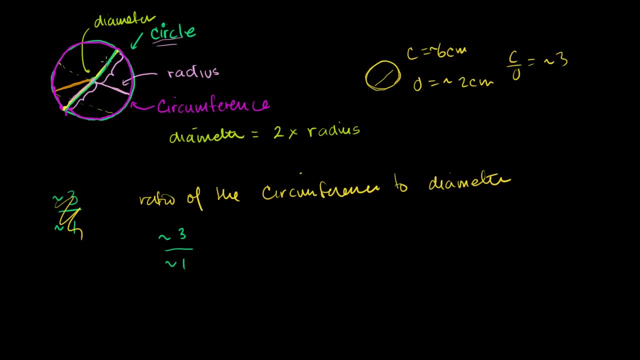 Maybe the ratio of the circumference to the diameter is always fixed for any circle. So they said: let me study this further. So they got better tape measures. And when they got better tape measures they measured: hey, you know, my diameter is definitely 1.. 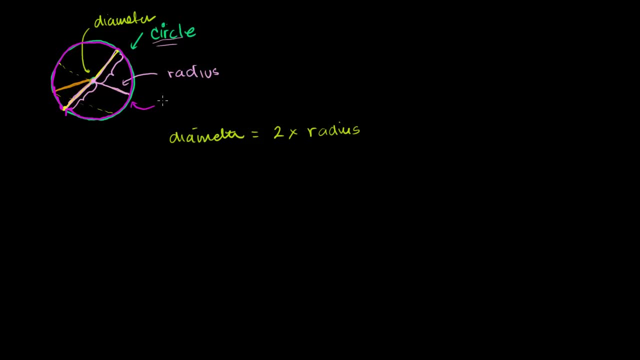 the circle like that. what's that distance? We call that word the circumference of the circle. Now we know how the diameter and the radius relates, But how does the circumference relate to, say, the diameter? If we know how it relates to the diameter, it's very easy. 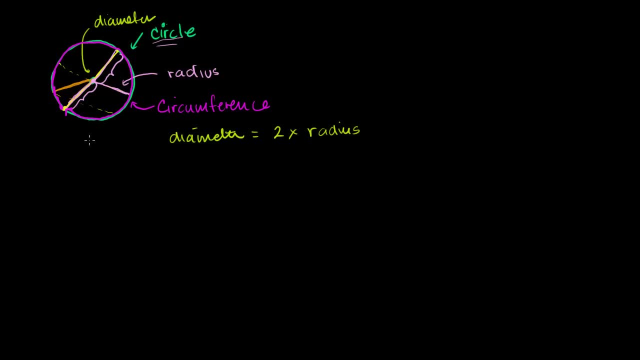 to figure out how it relates to the radius. Well, many thousands of years ago, people took their tape measures out And they keep measuring. They keep measuring circumferences and radiuses And, let's say, when their tape measures weren't so good. 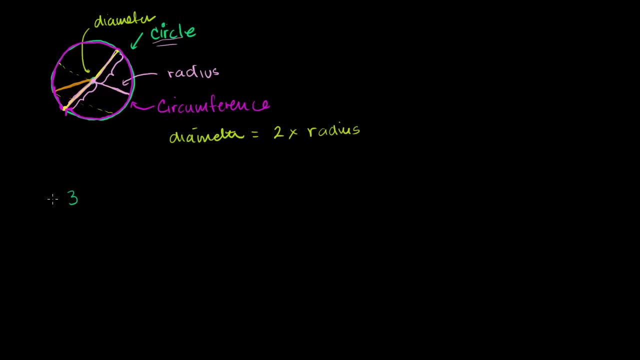 let's say they measured the circumference of the circle And they would get: well, it looks like it's about 3.. And then they measure the radius of this circle right here, or the diameter of that circle, And they'd say: well, that diameter looks. 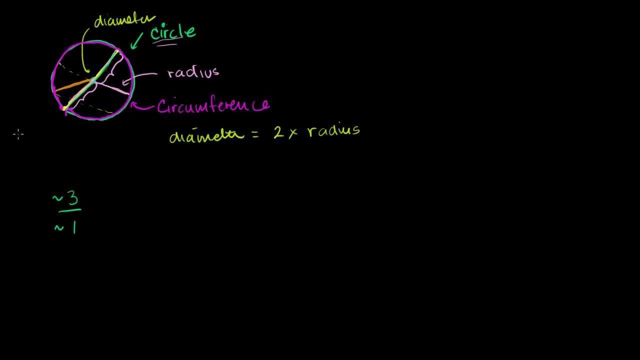 like it's about 1.. So they would say, let me write this down. So we're worried about the ratio of the circumference to the diameter. So let's say that somebody had some circle over here. Let's say they had this circle. 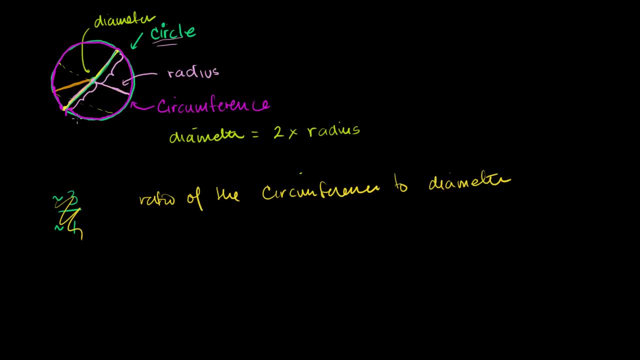 And the first time with not that good of a tape measure. they measured around the circle And they said: hey, it's roughly equal to 3 meters. when I go around it And when I measure the diameter of the circle, it's. 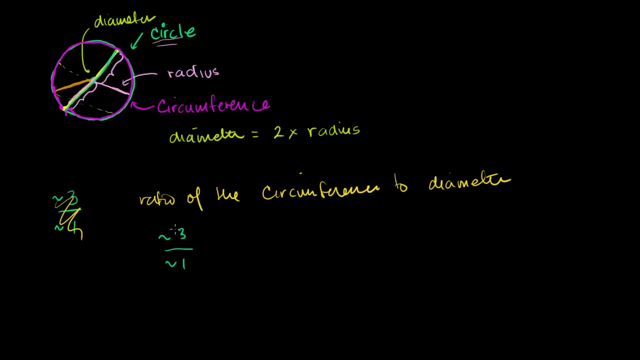 roughly equal to 1.. OK, that's interesting. It may be the ratio of the circle, The circumference of the diameter, is 3. So maybe the circumference is always 3 times the diameter. Well, that was just for this circle. 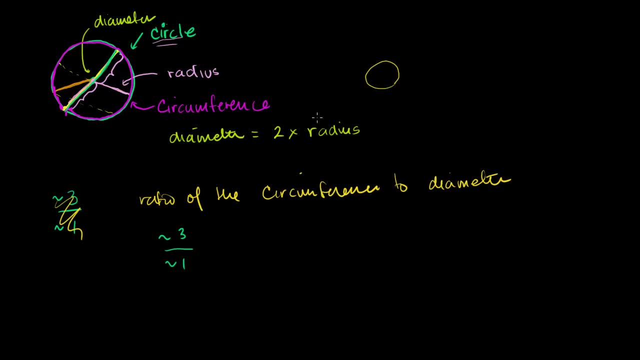 But then let's say they measured some other circle here. Let's say it's like this, I drew it smaller. But let's say that on this circle they measured around it and they found out that the circumference is 6 centimeters roughly. 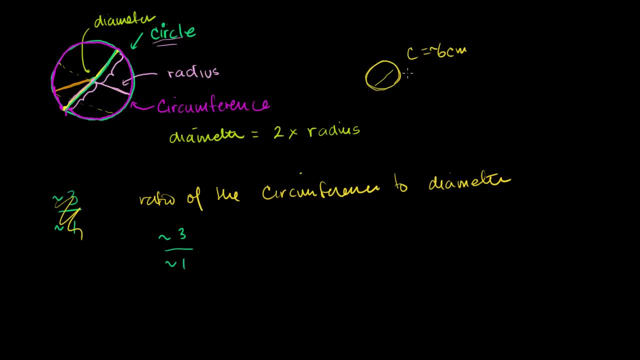 We have a bad tape measure right then. And then they find out that the diameter is roughly 2 centimeters And once again, the ratio of the circumference to the diameter, The circumference to diameter, was roughly 3.. OK, this is a neat property of circles. 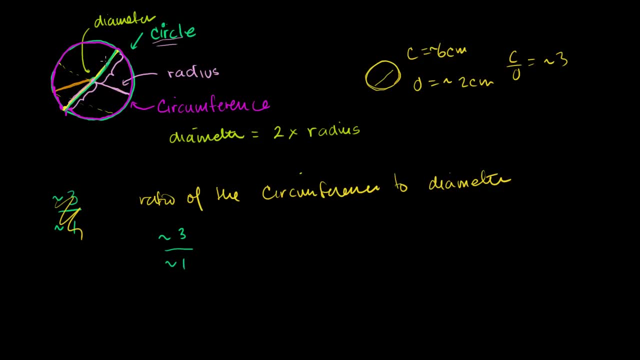 Maybe the ratio of the circumference to the diameter is always fixed for any circle. So they said: let me study this further. So they got better tape measures. And when they got better tape measures they measured: hey, you know, my diameter is definitely 1.. 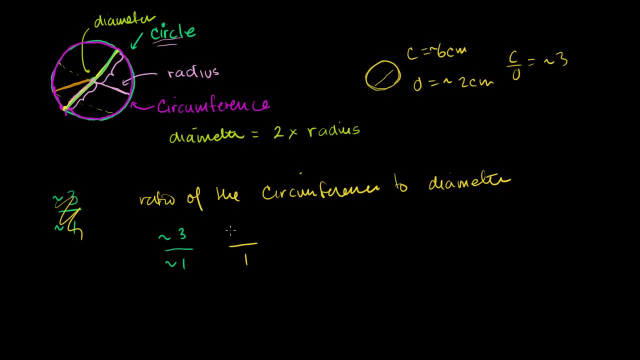 They say my diameter is definitely 1. But when I measure my circumference a little bit I realize it's closer to 3.1.. And the same thing with this Over here they noticed that this ratio is closer to 3.1.. 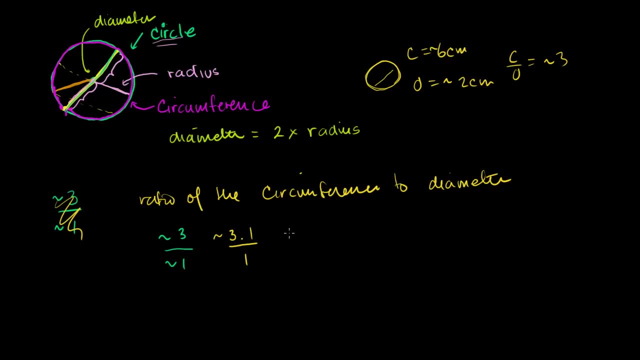 And then they kept measuring it better and better and better, And then they realized that they were getting this number. They just kept measuring it better and better and better, And they were getting this number: 3.14159.. And they just kept adding digits. 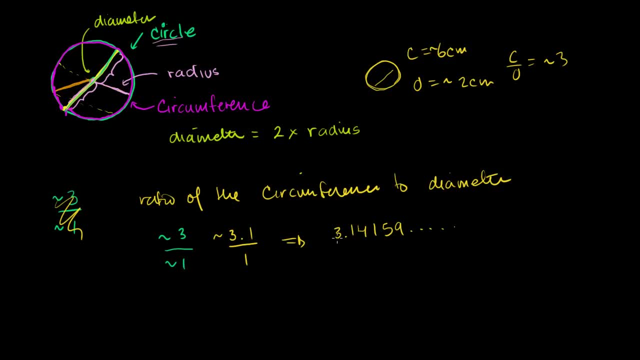 And it would never repeat. And it was this strange, fascinating, metaphysical number that kept showing up. And so, since this number was so fundamental to our universe, because a circle is so fundamental to our universe, and it just showed up for every circle, 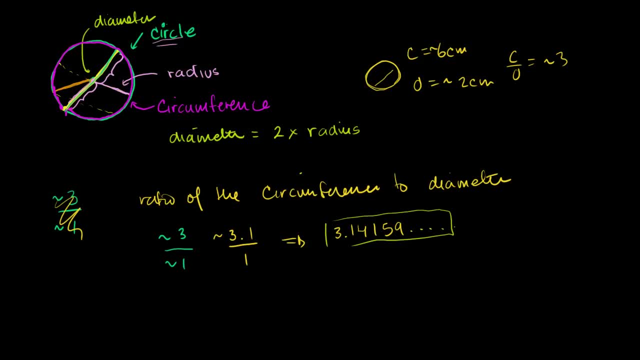 The ratio of the circumference to the diameter was this kind of magical number. They gave it a name. They called it pi, Or you could just give it the Latin or the Greek letter pi, Just like that. That represents this number, which is arguably the most. 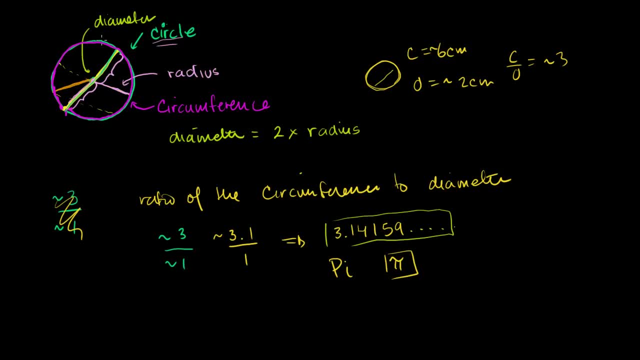 fascinating number in our universe. It first shows up as the ratio of the circumference to the diameter, but you're going to learn as you go through your mathematical journey that it shows up everywhere. It's one of these fundamental things about the universe that just makes you think that there's some order to it. 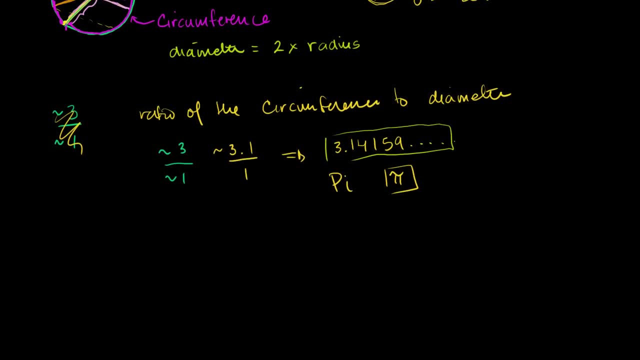 But anyway, how can we use this in our basic mathematics? So we know, or I'm telling you, that the ratio of the circumference to the diameter- When I say the ratio literally, I'm just saying if you divide the circumference by the diameter, you're going to. 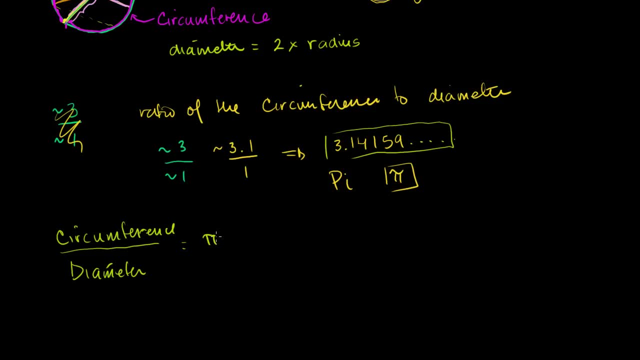 get pi. Pi is just this number. I could write 3.14159 and just keep going on and on and on, but that would be a waste of space and it would just be hard to deal with. So people just write this Greek letter, pi, there. 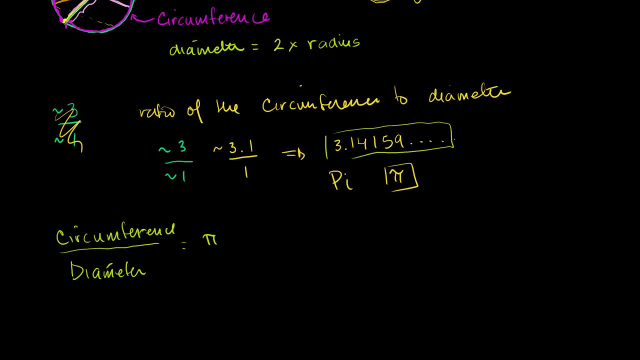 So how can we relate this? We can multiply both sides of this by the diameter and we could say that the circumference is equal to pi times the diameter. Or, since the diameter is equal to 2 times the radius, we could say that the circumference is equal to pi times the. 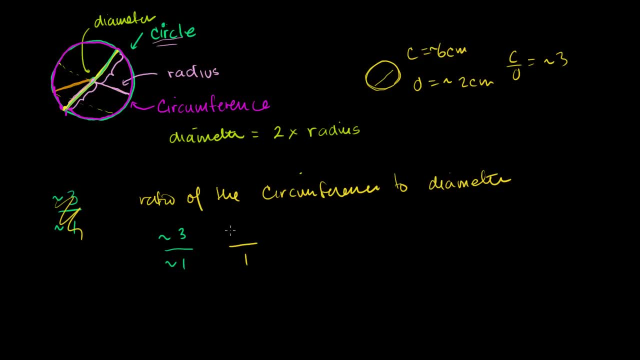 They say my diameter is definitely 1., But when I measure my circumference a little bit I realize it's closer to 3.1.. Closer to 3.1. And the same thing with this over here. They noticed that this ratio is closer to 3.1.. 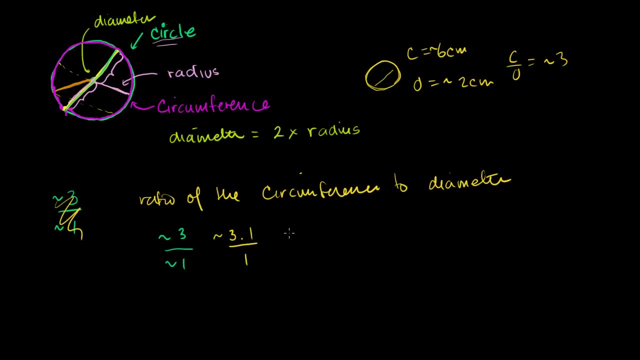 And then they kept measuring it better and better and better, And then they realized that they were getting this number. They just kept measuring it better and better and better And they were getting this number of 3.14159.. And they just kept adding digits. 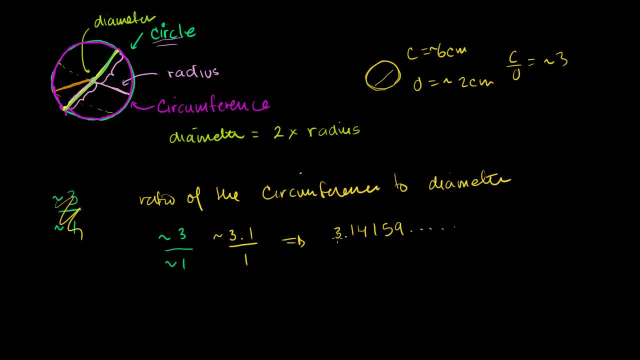 And it would never repeat. And it was this strange, fascinating, metaphysical number that kept showing up. And so, since this number was so fundamental to our universe- because a circle is so fundamental to our universe, and it just showed up, It just showed up. 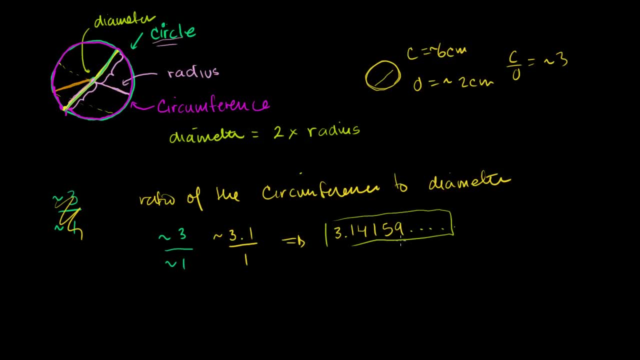 Every circle, the ratio of the circumference to the diameter was this kind of magical number. They gave it a name. They called it pi, Or you could just give it the Latin or the Greek letter pi. Just like that, That represents this number, which is arguably the most. 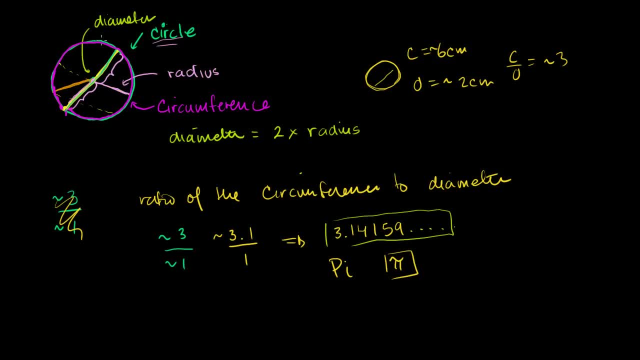 fascinating number in our universe. It first shows up as the ratio of the circumference to the diameter, but you're going to learn as you go through your mathematical journey. It shows up everywhere. It's one of these fundamental things about the universe that just makes you think that there's some order to it. 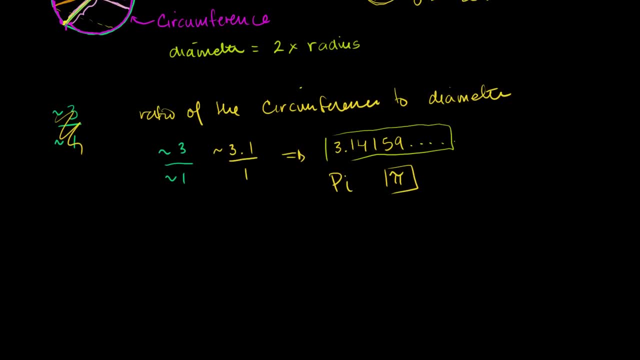 But anyway, how can we use this in our basic mathematics? So we know, or I'm telling you that the ratio of the circumference to the diameter. When I say the ratio literally, I'm just saying if you divide the circumference by the diameter. 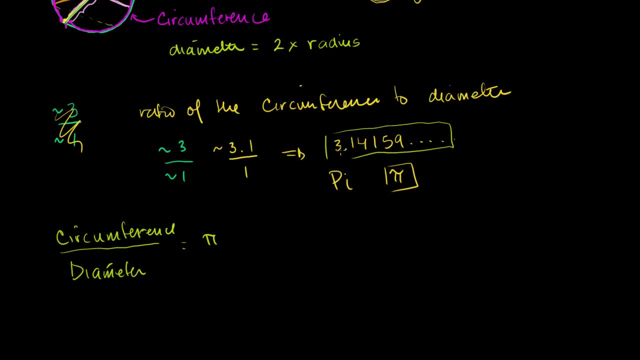 You're going to get pi. Pi is just this number. I could write 3.14159 and just keep going on and on and on, but that would be a waste of space and it would just be hard to deal with. So people just write this Greek letter, pi, there. 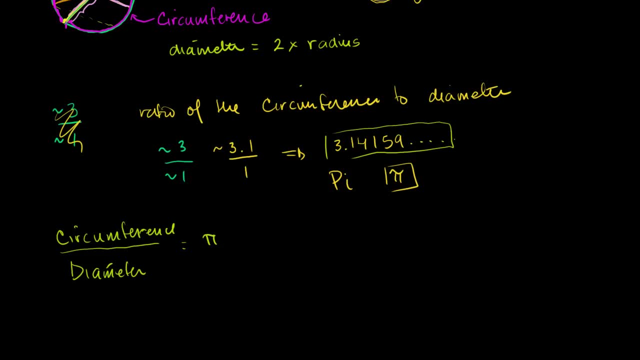 So how can we relate this? We can multiply both sides of this by the diameter and we could say that the circumference is equal to pi times the diameter. Or, since the diameter is equal to 2 times the radius, we could say that the circumference is equal to pi times 2 times the. 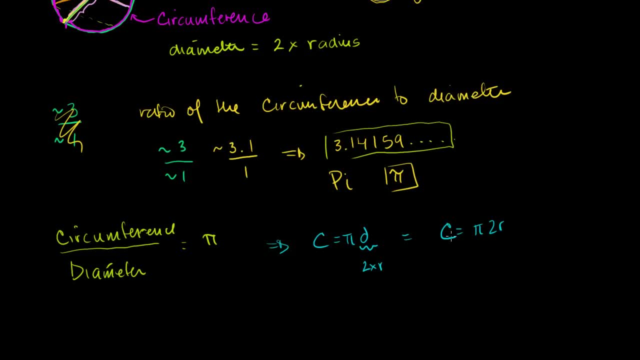 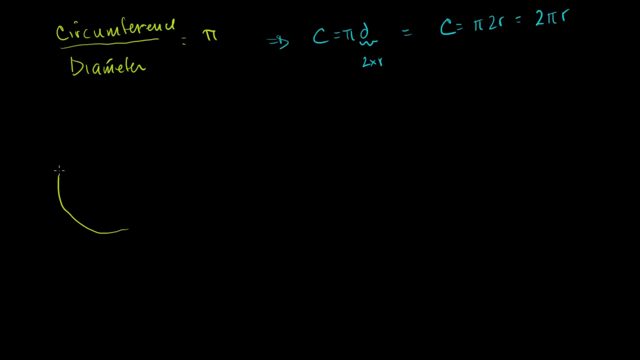 radius Or the form that you're most likely to see it, it's equal to 2 pi r. So let's see if we can apply that to some problems. So let's say: I have a circle, I have a circle, just like that. 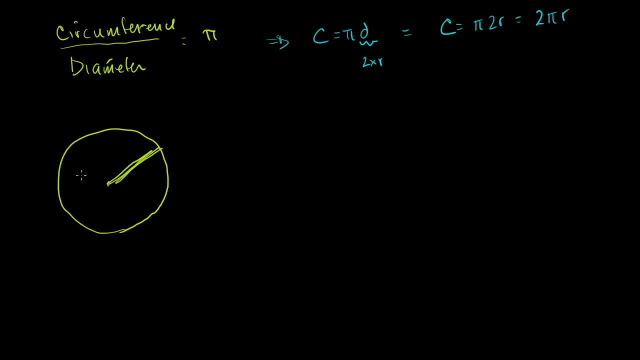 And I were to tell you it has a radius. Its radius, right there, is 3.. So 3, let me write this down. So the radius Is equal to 3.. Maybe it's 3 meters. Put some units in there. 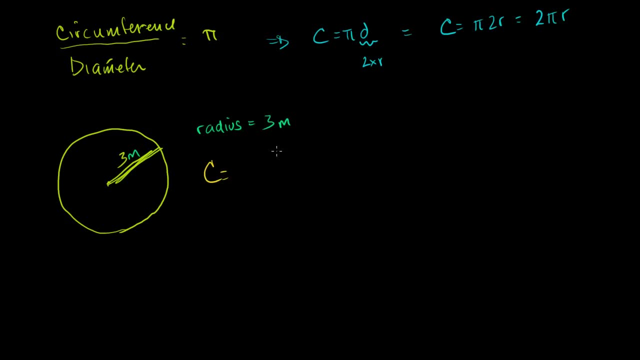 What is the circumference of this circle? The circumference is equal to 2 times pi times the radius, So it's going to be equal to 2 times pi times the radius Times 3 meters, Which is equal to 6 meters times pi, or 6 pi meters. 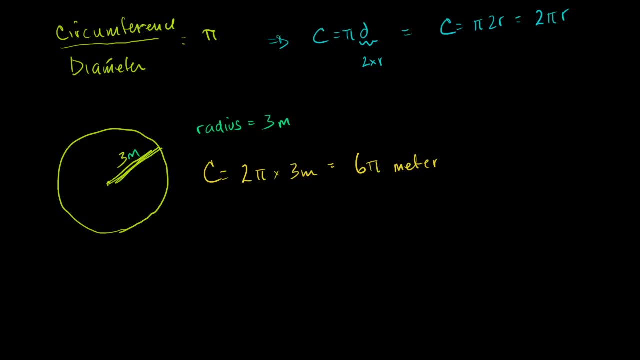 Now I could multiply this out. Remember, pi is just a number, Pi is 3.14159, going on and on and on. So if I multiply 6 times that, maybe I'll get 18, point something, something, something. 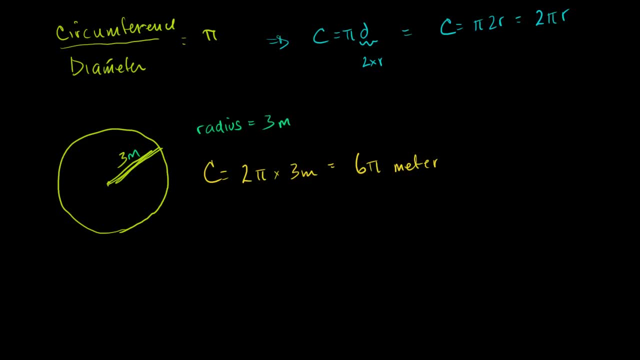 If you have your calculator you might want to do it, But for simplicity people just tend to leave our numbers in terms of pi. I don't know what this is If you multiply 6 times 3.14159,. I don't know if you. 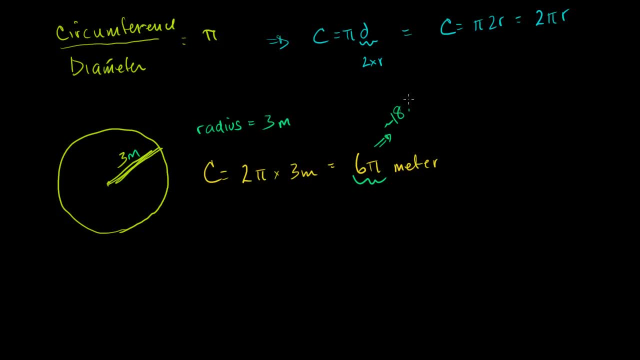 get something close to 19 or 18.. Maybe it's approximately 18 point something, something, something. I don't have my calculator in front of me, But instead of writing that number, you just write 6.14159.. 6 pi there. 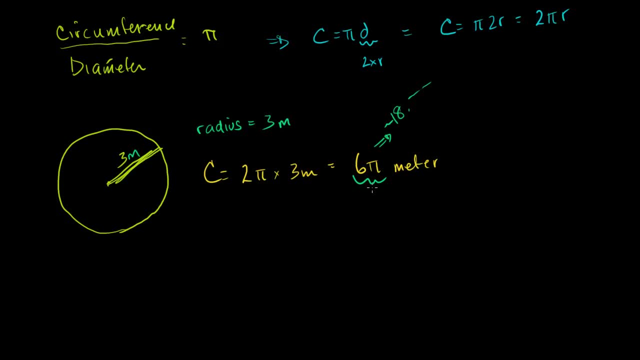 Actually, I think it wouldn't quite cross the threshold to 19 yet. Now what if I were to go there? Well, let's ask another question: What is the diameter of this circle? What is the diameter? Well, if this radius is 3,, the diameter is just twice that. 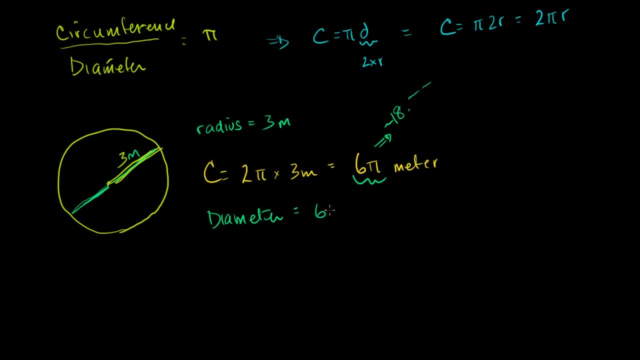 So it's just going to be 3 times 2, or 3 plus 3,, which is equal to 6 meters. So the circumference is 6 pi meters, The diameter is 6 meters, The radius is 3 meters. 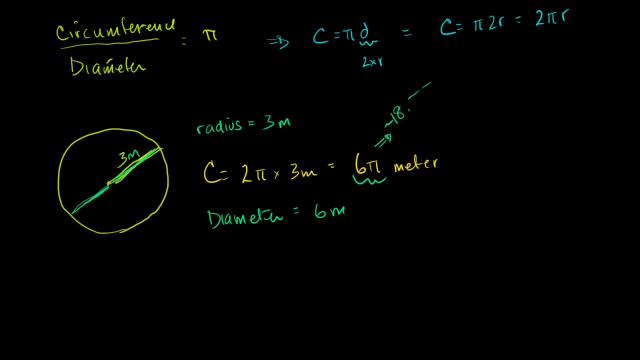 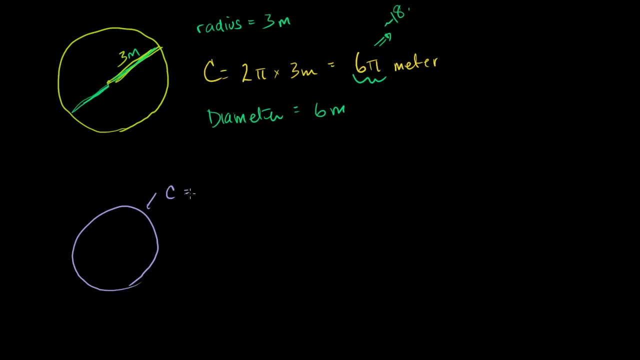 Now let's go the other way. Let's say I have another circle. Let's say I have another circle here And I were to tell you that its circumference, the circumference, is equal to 10 meters. That's the circumference of the circle. if you were to put 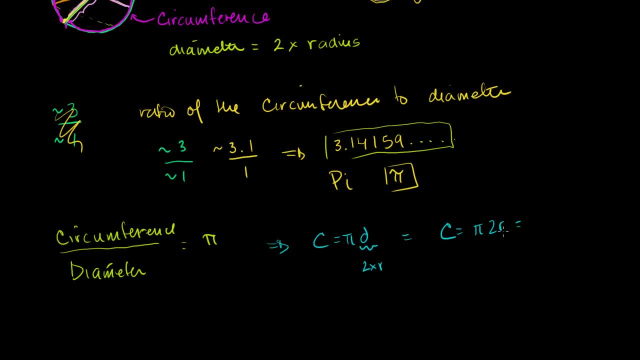 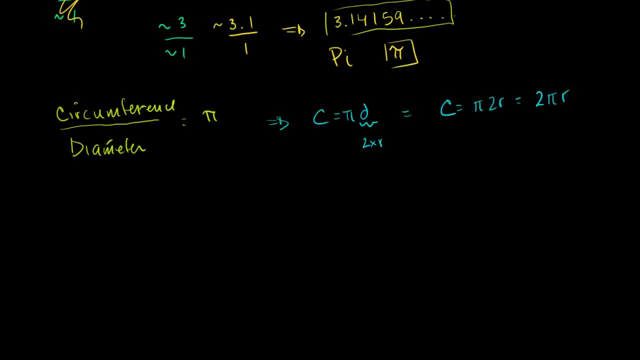 radius or the form that you're most likely to see it, It's equal to 2 pi r. So let's see if we can apply that to some problems. So let's say: I have a circle, I have a circle, just like that. 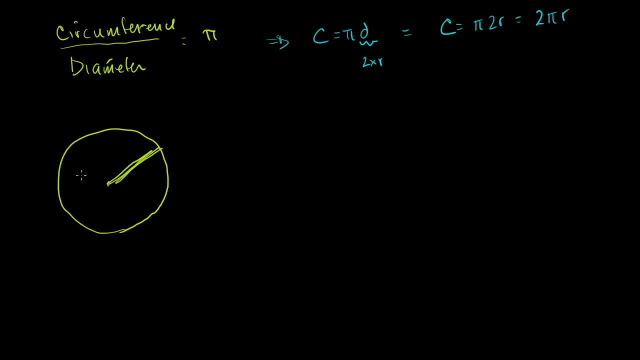 And I were to tell you it has a radius. Its radius, right there, is 3.. So 3, let me write this down. So the radius Is equal to 3.. Maybe it's 3 meters. Put some units in there. 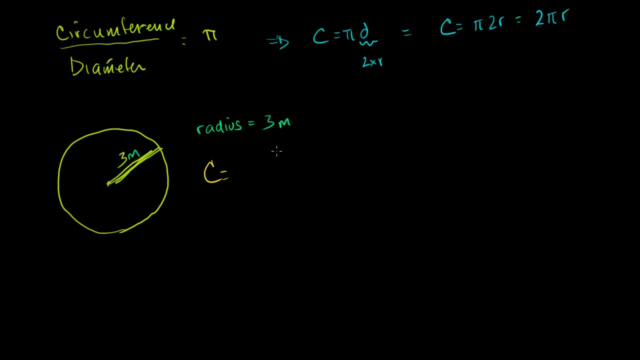 What is the circumference of the circle? The circumference is equal to 2 times pi times the radius. So it's going to be equal to 2 times pi times the radius times 3 meters, which is equal to 6 meters times pi, or 6 pi. 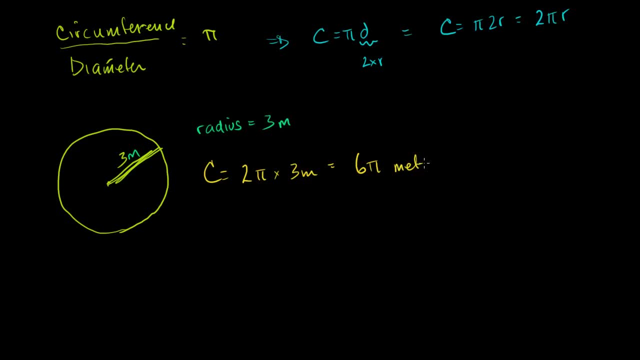 meters. Now I could multiply this out. Remember, pi is just a number. Pi is 3.14159,. going on and on and on. So if I multiply 6 times that, maybe I'll get 18 point. something, something, something. 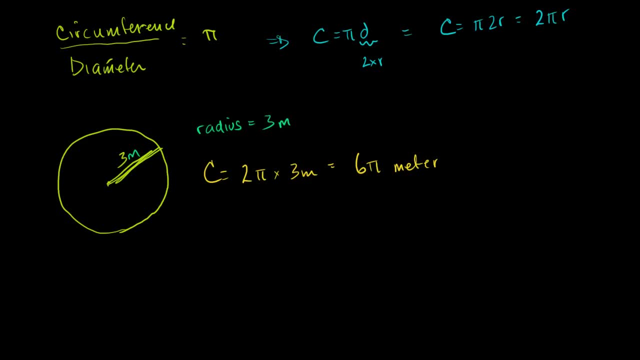 If you have your calculator you might want to do it, But for simplicity people just tend to leave our numbers in terms of pi. I don't know what this is If you multiply 6 times 3.14159,. I don't know if you. 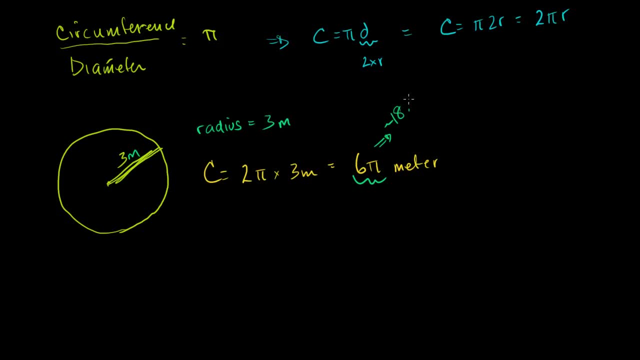 get something close to 19 or 18.. Maybe it's approximately 18 point something, something, something. I don't have my calculator in front of me, But instead of writing that number, you just write: oh, I'm going to do this. 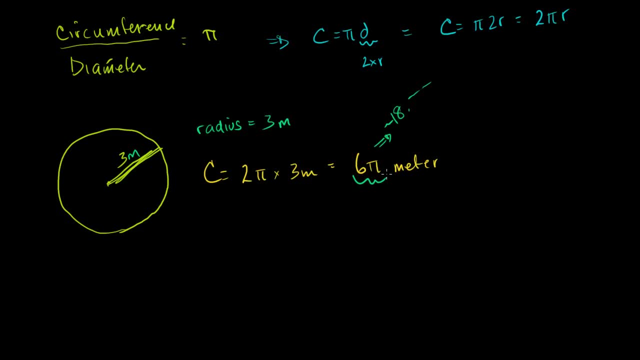 You just write 6 pi there. Actually, I think it wouldn't quite cross the threshold to 19 yet. Now what if I were to go there? Well, let's ask another question: What is the diameter of the circle? What is the diameter? 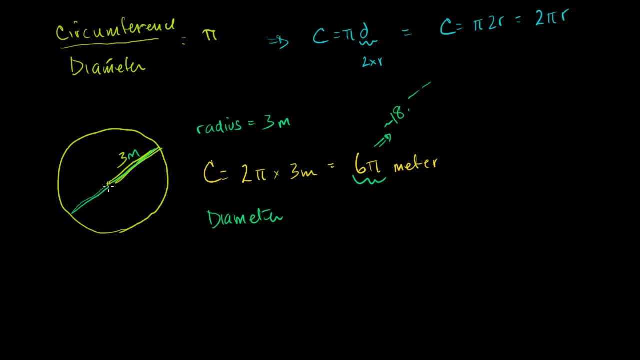 Well, if this radius is 3,, the diameter is just twice that. So it's just going to be 3 times 2, or 3 plus 3,, which is equal to 6 meters. So the circumference is 6 pi meters. 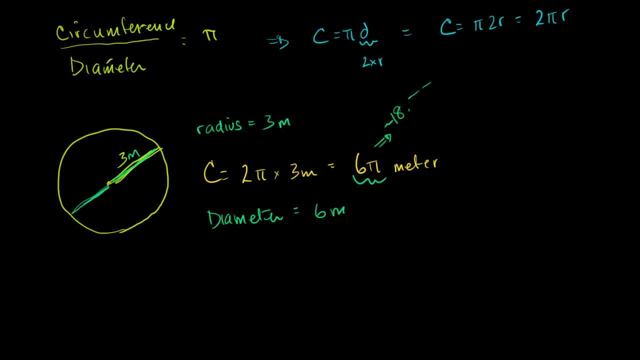 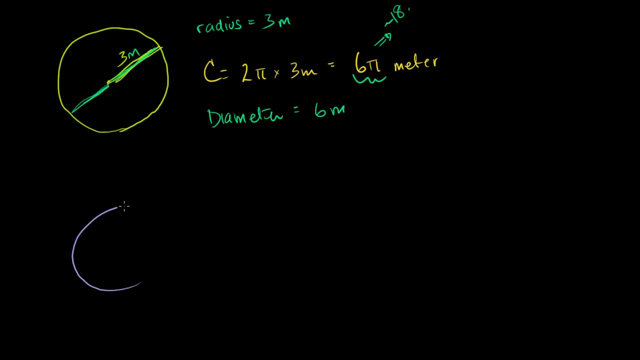 The diameter is 6 meters, The radius is 3 meters. Now let's go the other way. Let's say I have another circle. Let's say I have another circle here And I were to tell you that its circumference is equal to. 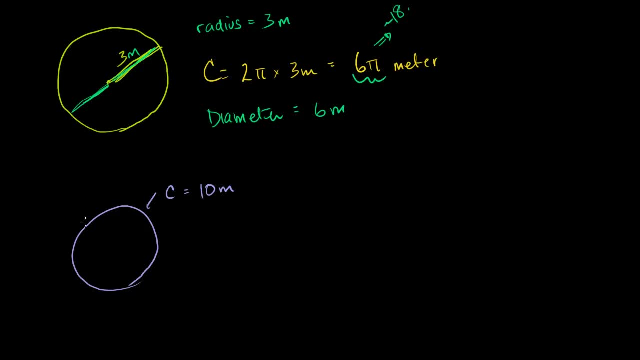 10 meters. That's the circumference of the circle. if you were to put a tape measure to go around it And someone were to ask you what is the diameter of the circle, Well, we know that the diameter times pi. We know that pi times the diameter. 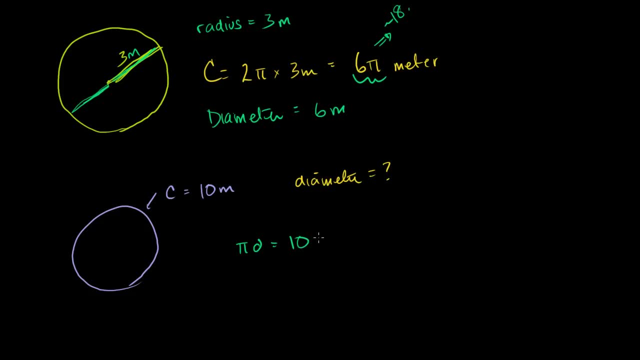 Is equal to the circumference Is equal to 10 meters. So to solve for this, we would just divide both sides of this equation by pi, So the diameter would equal 10 meters over pi or 10 over pi meters, And that is just a number. 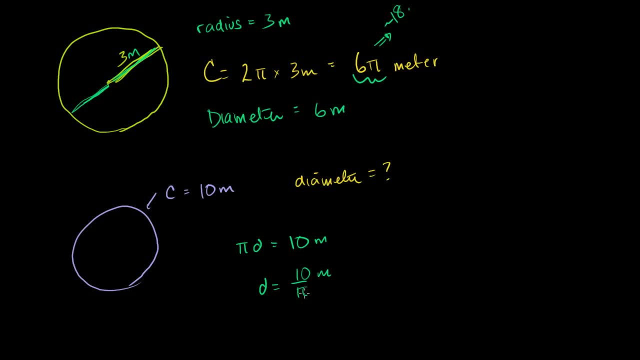 If you have your calculator, you could actually divide 10 divided by 3.14159.. You're going to get 3 point something. something meters. I can't do it in my head, But this is just a number. But for simplicity we often just leave it that way. 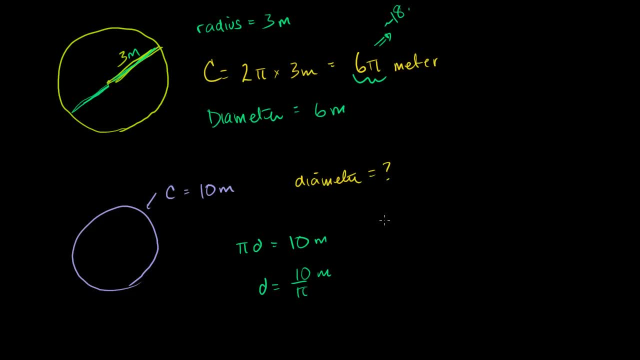 Now, what is the diameter of the circle? Well, the radius is equal to 1 half the diameter. So this whole distance right here is 10 over pi meters. And if we would just want half of that, if we just want the. 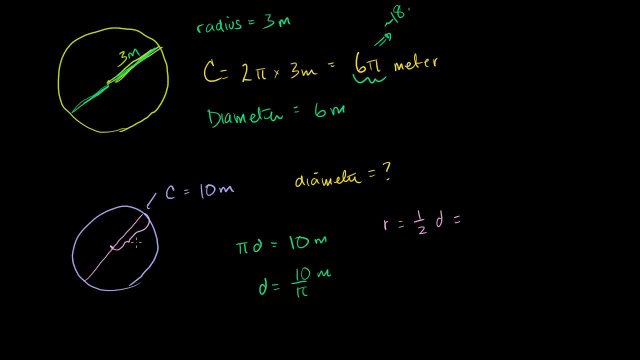 radius. we just multiply it times half, So you have 1 half times 10 over pi, which is equal to 1 half times 10, or you could just divide the numerator and the denominator by 2. You get a 5 there. 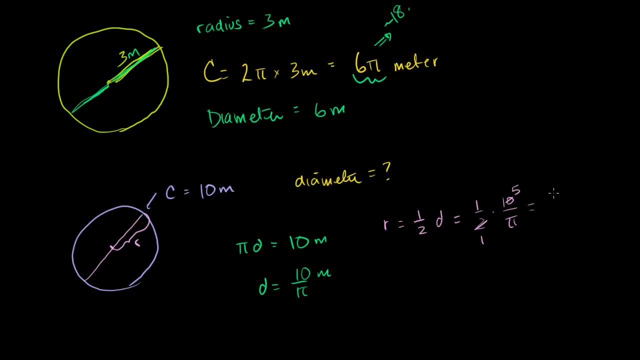 So you get 5 over pi. So the radius over here is equal to 1 half the diameter. OK, Over here is 5 over pi. Nothing super fancy about this. I think the thing that confuses people the most is to just 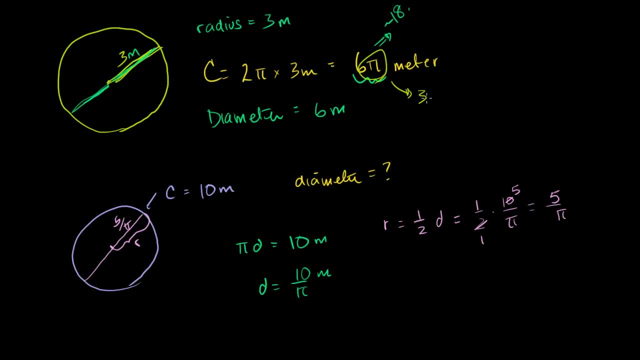 realize that pi is a number. Pi is just 3.14159.. It just keeps going on and on and on. There's actually thousands of books written about pi, So it's not like you know. I don't know if there's. 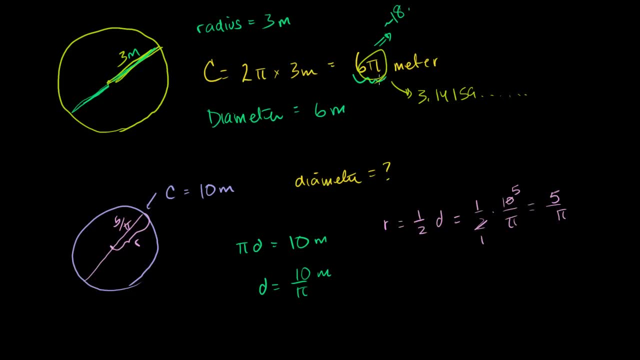 thousands, but maybe I'm exaggerating. But you could write books about this number, But it's just a number. It's a very special number And if you wanted to write a number, you could write a, write it in a way that you're used to writing numbers. 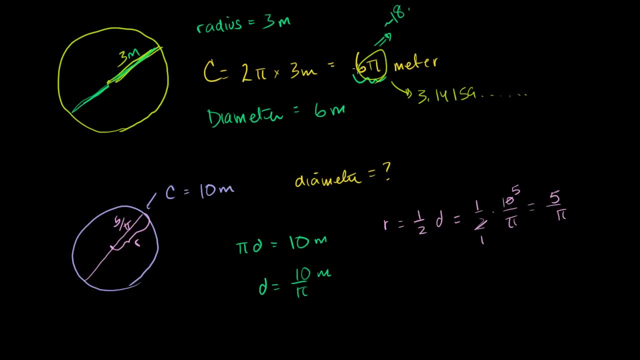 You could literally just multiply this out, But most of the time people just realize they like leaving things in terms of pi. Anyway, I'll leave you there And in the next video we'll figure out the area of a circle. 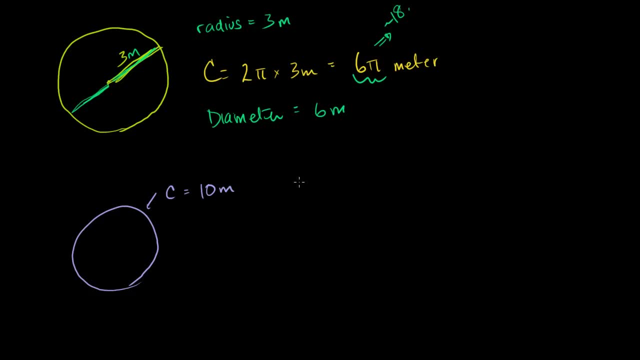 a tape measure to go around it And someone were to ask you what is the diameter of the circle? Well, we know that the diameter times pi. we know that pi times the diameter is equal to the circumference. So the diameter is equal to 10 meters. 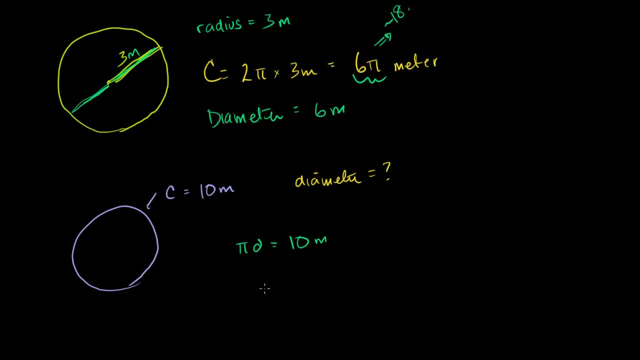 So to solve for this, we would just divide both sides of this equation by pi, So the diameter would equal 10 meters over pi or 10 over pi meters, And that is just a number. If you have your calculator, you could actually divide 10. 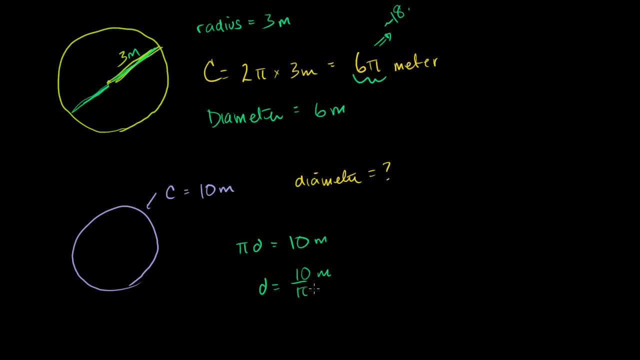 divided by 3.14159.. You're going to get 3 point something, something, something. meters. I can't do it in my head, But this is just a number, But for simplicity we often just leave it that way. Now, what is the radius? 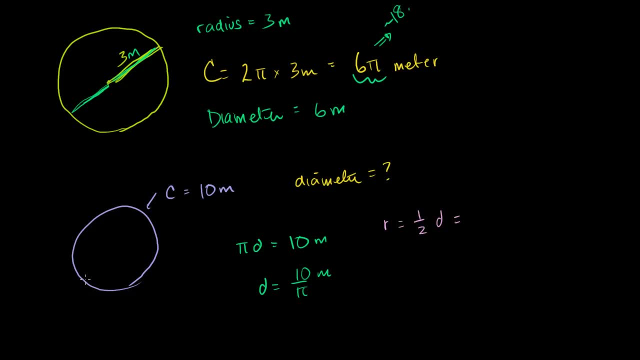 Well, the radius is equal to 1 half the diameter. So this whole distance right here is 10 over pi meters. And if we would just want half of that, if we just want the radius, we just multiply it times half. So you have 1 half times 10 over pi, which is equal to 1. 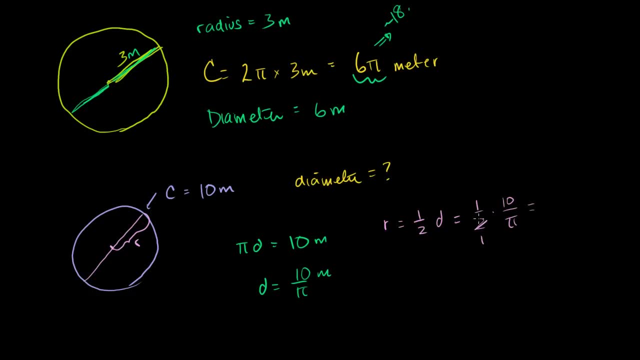 half times 10.. Or you could just divide the numerator and the denominator by 2. You get a 5 there. So you get 5 over pi. So the radius over here is 5 over pi. Nothing super fancy about this. 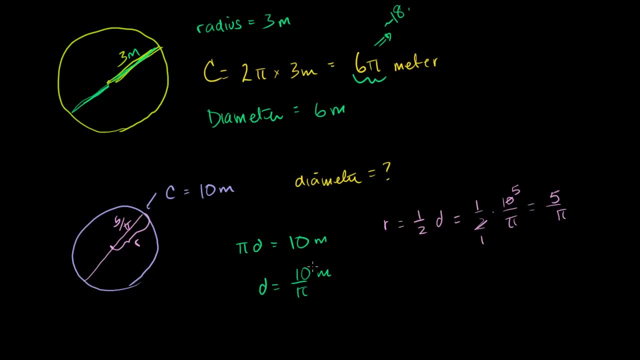 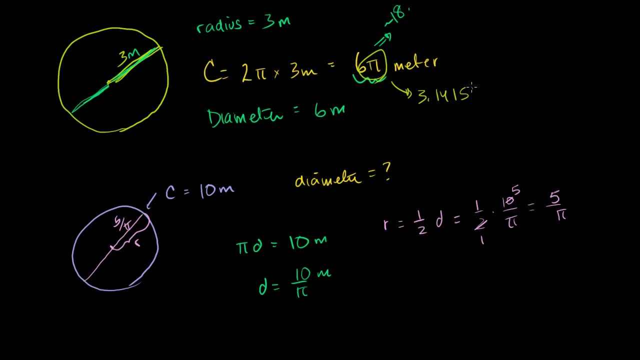 just realize that pi is a number. Pi is just 3.14159.. It just keeps going on and on. You could write there's actually thousands of books written about pi. So it's not like I don't know if there's thousands. but 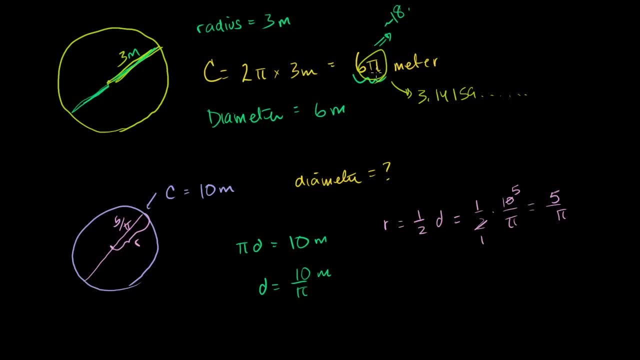 maybe I'm exaggerating, But you could write books about this number. But it's just a number. It's a very special number And if you wanted to write it in a way that you're used to out, but most of the time people just realize they like 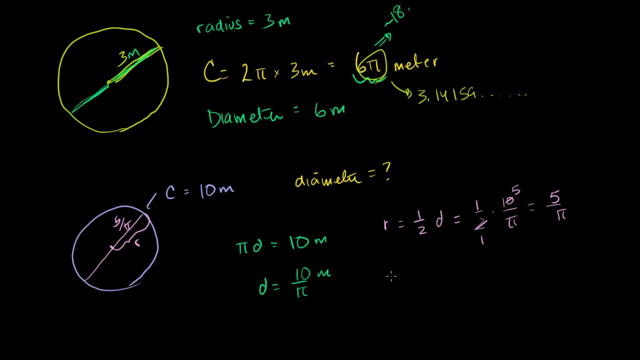 leaving things in terms of pi. Anyway, I'll leave you there and in the next video we'll figure out the area of a circle.